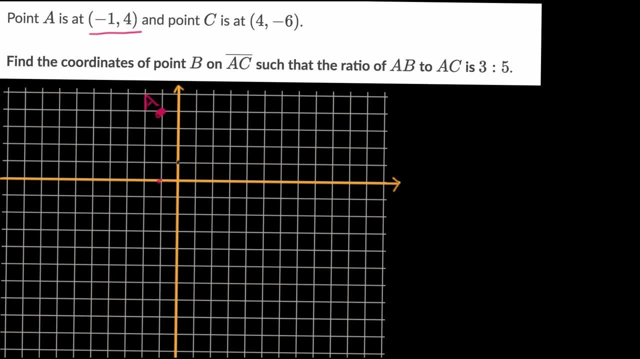 So that right over there is point A, And then let's think about point C, which is at four comma negative six. So one, two, three, four comma negative, six Negative, one negative, two negative, three negative, four negative, five negative six. 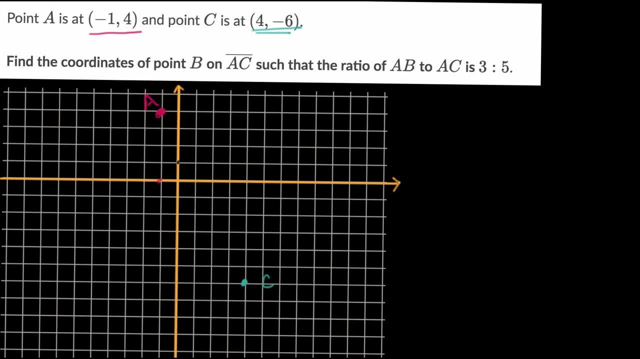 Just like that. And so the segment AC. I get my ruler tool out here. Segment AC is going to look like that, And the ratio between the distance of A to B and A to C is three to five, Or another way to think about it is. 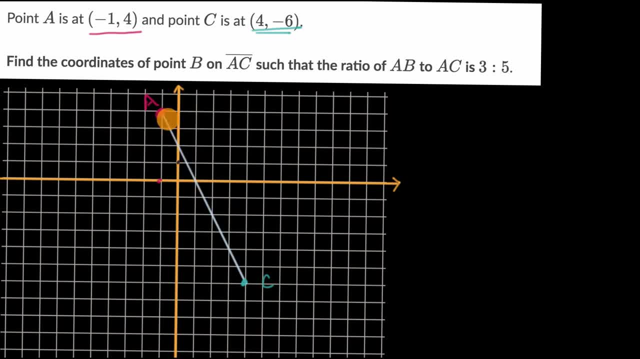 B is going to be three fifths along the way from A to C. Now, the way that I think about it is, in order to be three fifths along the way from A to C, you have to be three fifths along the way in the X direction. 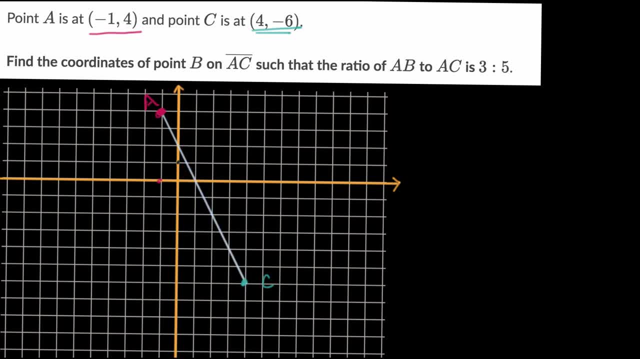 and three fifths along the way in the Y direction. So let's think about the X direction first. We are going from X equals negative one to X equals four. to go from this point to that point, Our change in X is one, two, three, four, five. 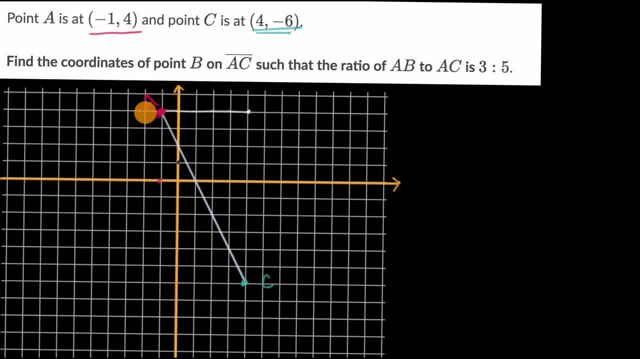 And so if we want to go three fifths of that, we went a total of five. Three fifths of that is going just three. So that is going to be B's X squared, And then we can look on the Y coordinate side. 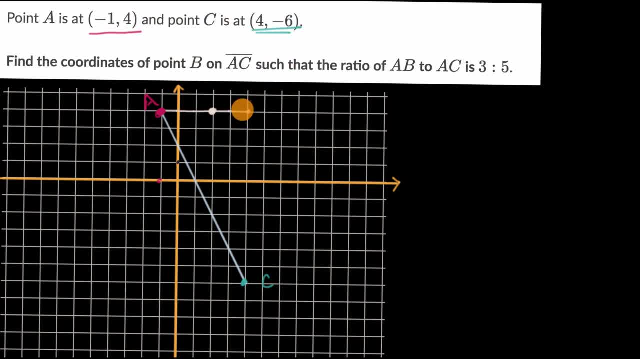 To go from A to C, we are going from four to negative six. So we're going down by one, two, three, four, five, six, seven, eight, nine, 10.. And so three fifths of 10 would be six. 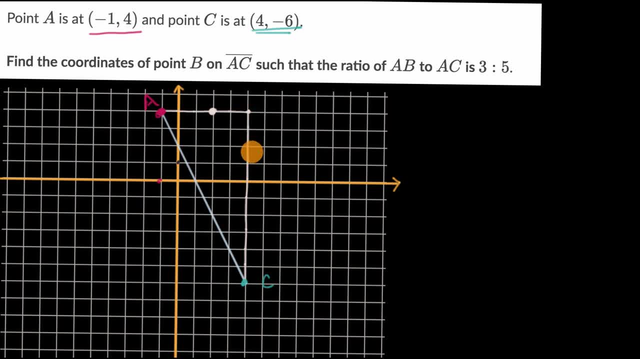 So B's coordinate is going to be one, two, three, four, five, six down. So just like that, we were able to figure out the X and the Y coordinates for point B, which would be right over here And you could look at this directly and say: 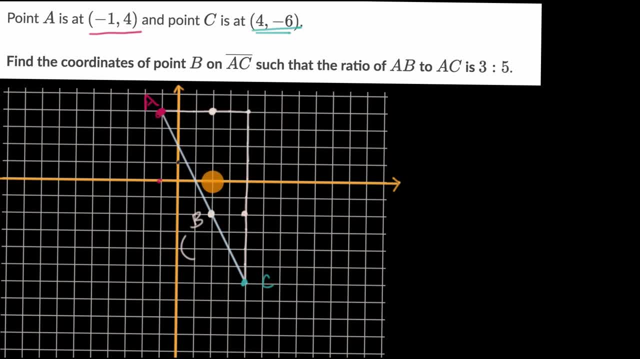 look, B is going to have the coordinates. This looks like this is two comma negative two, which we were able to do with the graph paper. So another way you could think about it, even algebraically, is the coordinates of B. we could think about it as starting with the coordinates.